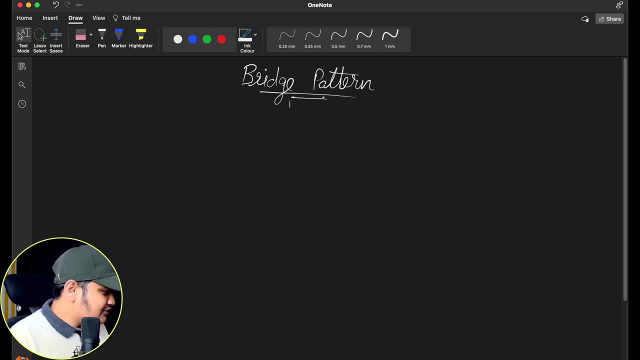 can see the video in the Netflix you can see the videos. So let's take that example. So currently you can see I have the video object here, video class, and this video class, you can see, I can divide into multiple classes. Suppose I can say this is a YouTube video. 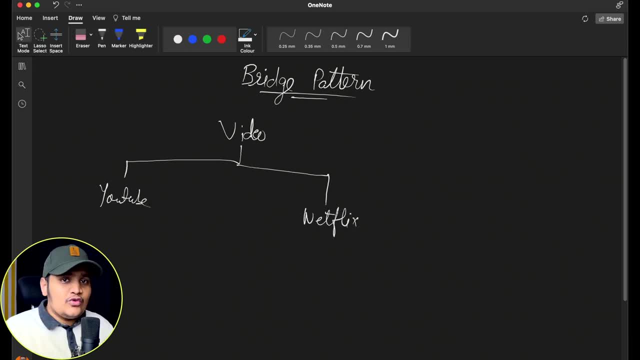 I can say: this is a Netflix video And within the YouTube and Netflix, you have different options as well. You can play the video in HD, 4K, 8K, Same with Netflix as well. So what you will do is, if you want to have. 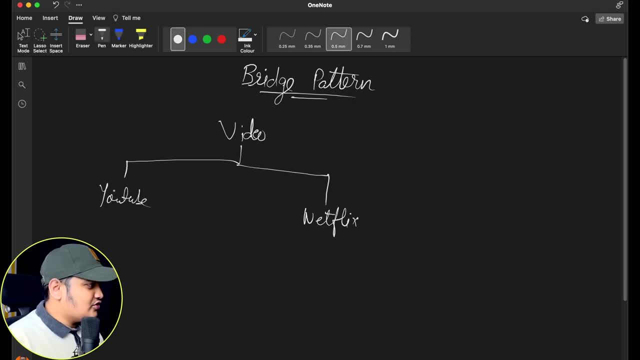 that functionality. you will create these subclasses, subtypes of that as well, So you can create YouTube with HD. You can create YouTube with 4K. You can create YouTube with 8K. Similarly, you can create Netflix with 4K and Netflix with 8K. 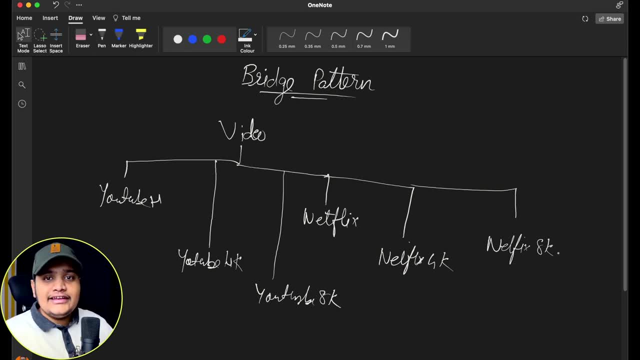 So you can see that by just adding the different type you are exponentially increasing the subclasses. suppose now, if you are introducing the prime video as well, so for that as well you will be adding the different subclasses like prime video HD, prime video 4k, prime video 8k and so on. so you can see: 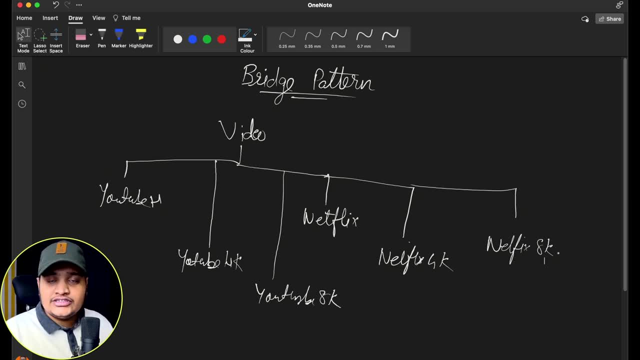 that whenever you are onboarding anything, you are creating a huge list of subclasses. so that is not ideal. you are just creating the classes exponentially. so what we can do to avoid that? okay, so at that time, bridge pattern comes into picture. so what bridge pattern will allow us to do is it will allow us to convert this entire user relationship. 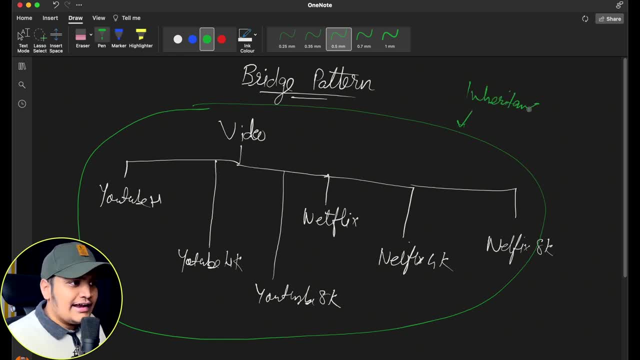 right. this is the entire user relationship. that is the inheritance right. it will allow us to convert this entire into a composition that is a has a relationship. so let's understand how this entire thing can be converted into the has a relationship. so let's take the example. 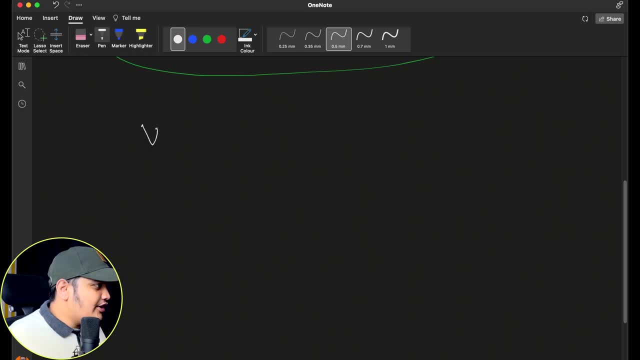 here. okay, so what I will have is I will have the video here, okay, video class, and this video class will have YouTube here and it has Netflix here. okay, you can see that. we have the simple hierarchy and, if I want, I can add the prime video as well here. so you can see that I have 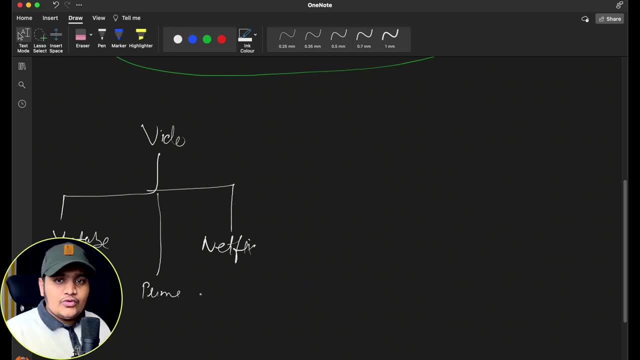 the standard classes available. here and now. what I want to do is I want to separate out the hierarchy right because I want to convert the inheritance into the composition relationship. so what I will do is, rather than creating the HD YouTube, 4k YouTube and similarly, I 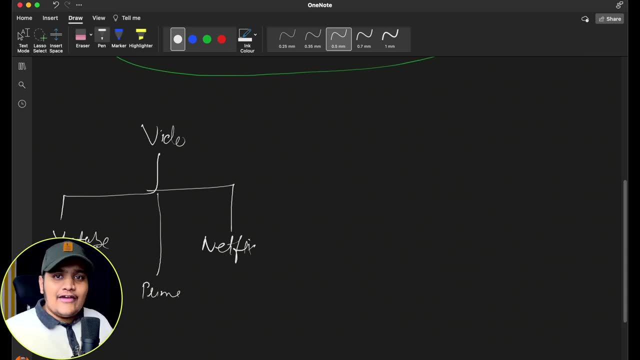 will create the processing classes separately and I will create the processing classes separately and I will create the has a relationship. so you can see that I can completely create a new hierarchy. that is the video processor and this video processor, you can see it has HD processor, it has 4k processor, it has 8k processor, it can have HDR or whatever it is. 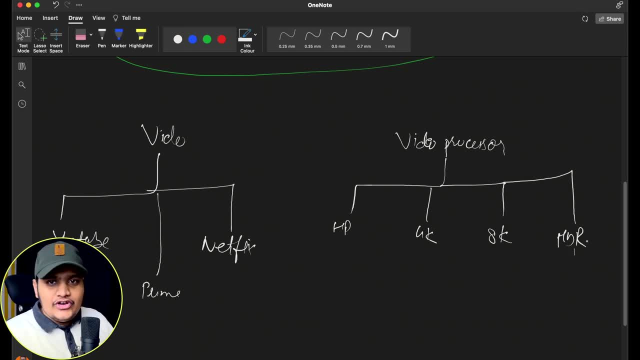 okay, so you can see that we have this processing available as a video processor. now what we will do is we will have the composition relationship. okay for this video. that this video will contain the video process processor. okay, so now video will have the relationship with the video processor. that. 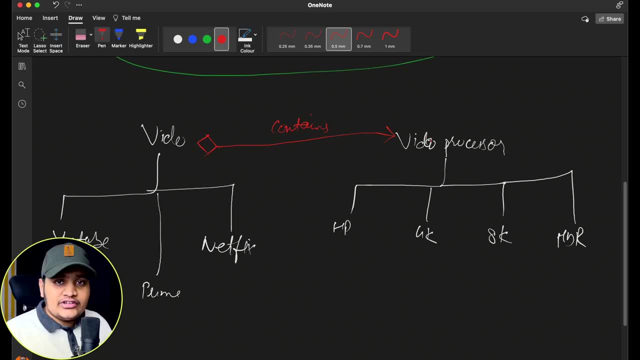 video will contain the video processor. so whenever we want to create the processing for a different pipeline for the different types of videos, we can do similarly, like for a youtube video. i can have the object of a video processor and i can create youtube video with hd, youtube video with 4k youtube. 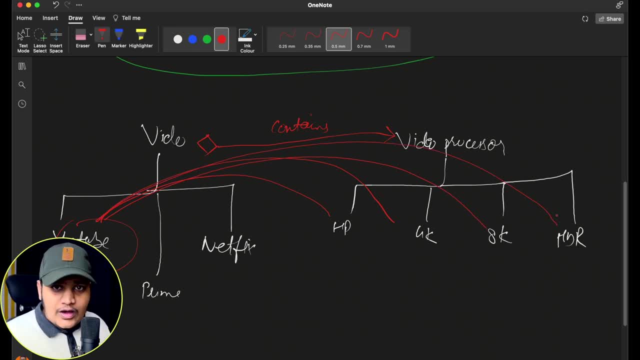 video with 8k. similarly, youtube video with hdr as well. similarly for netflix as well, i can do the same thing: netflix hd, netflix 4k, netflix 8k, similarly netflix hdr as well. so you can see that i am not creating the complete hierarchy, but i have the two separate hierarchy and i can create. 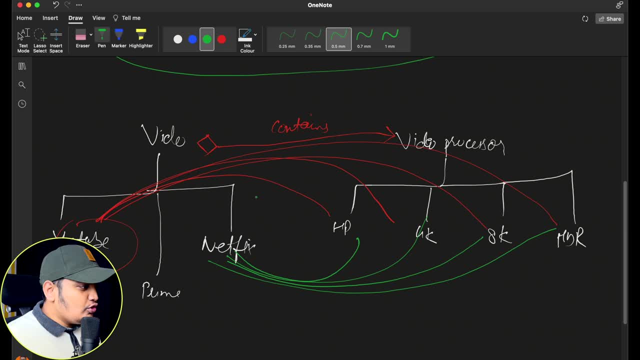 the objects, which has the contains relationship. okay, so whenever i want to create the object, that netflix object with the 4k, i can create it easily. so this is the general idea about the bridge design button, as this video processor, which is the instance available within this video, will work. 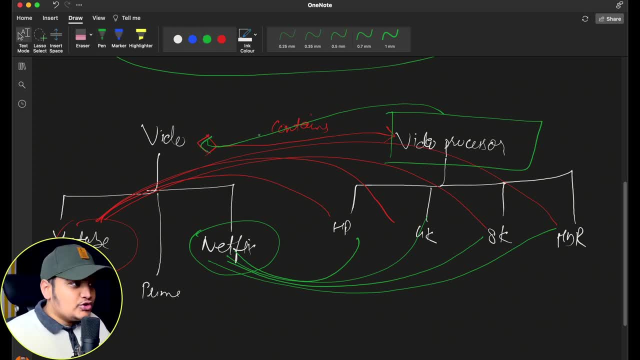 as a bridge between that and the video processor. okay, so that's why this is known as a bridge design pattern, because it's working as a bridge to have the different of the video classes itself, okay, like video hd, 4k, 8k and hdr. similarly. 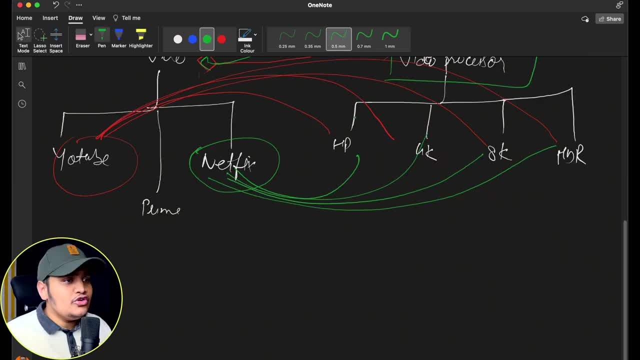 others as well. now, this is the simplest example that i have shown you. when you go through online, you will get more complex examples as well. okay, but if you want to understand the theoretical part as well, i will include the theoretical part in my code as well, okay, so let's understand with. 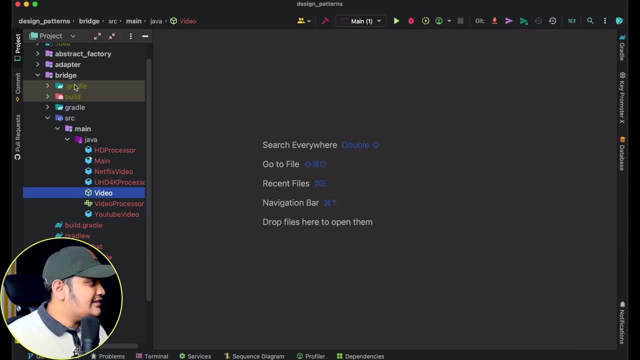 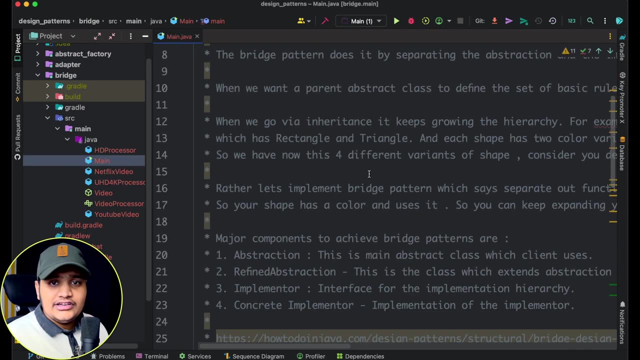 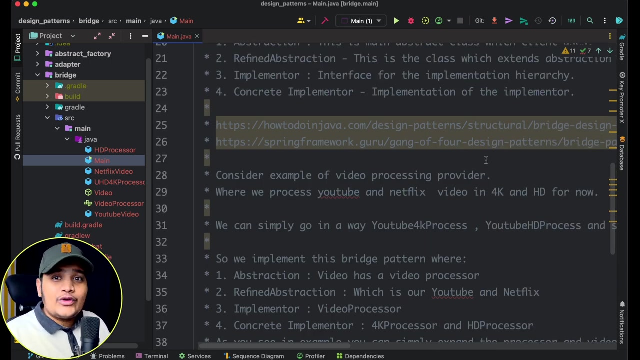 the code. so if we go to the intelligent idea here, okay, this is the bridge pattern, this will be available in the repository and if you go to the main method, you can see that entire documentation, entire theoretical part i have mentioned here, okay, and i've also mentioned from where i have taken the references so you can go through their websites and you can. 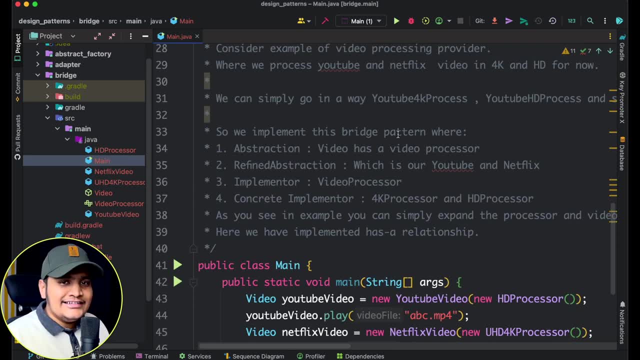 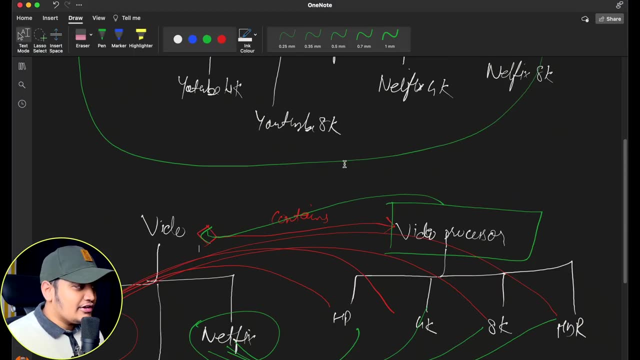 support them as well. so all this implementation, all these details are available here. let's understand, with the video here, how this will work. so whatever we explained here, whatever we understood here, the similar thing we have created here as well. so you can see that we have the video interface. 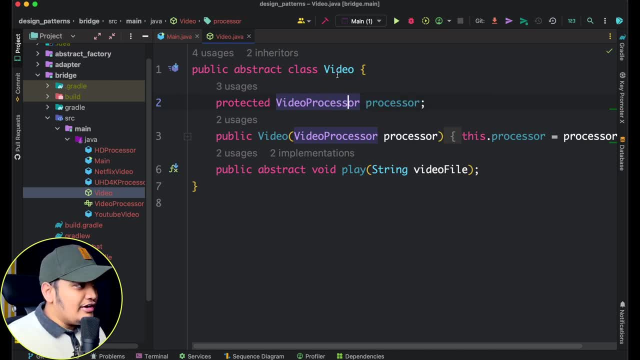 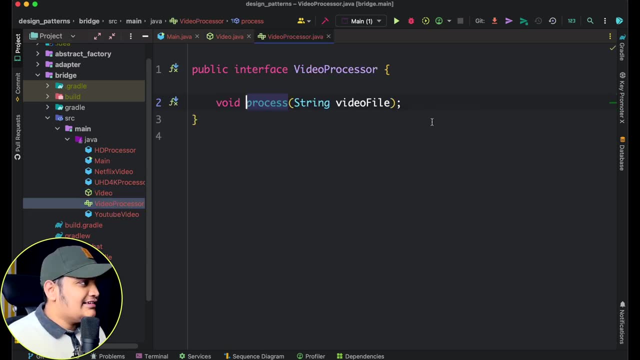 created abstract class or the same thing. here. we don't have to create the same thing again, so let's class. sorry, so you can see this video class: this is the hierarchy 1, and video processor: this is the hierarchy 2. so if you go to the video processor here, right, this is the another interface and this: 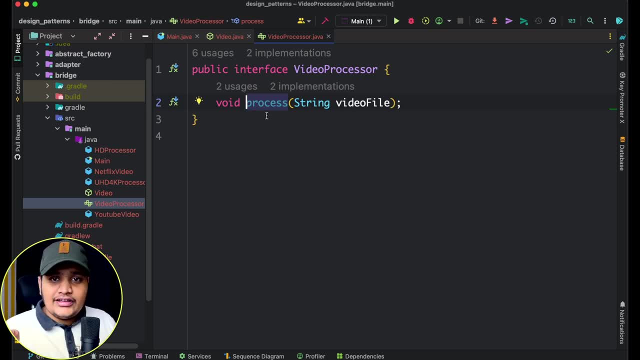 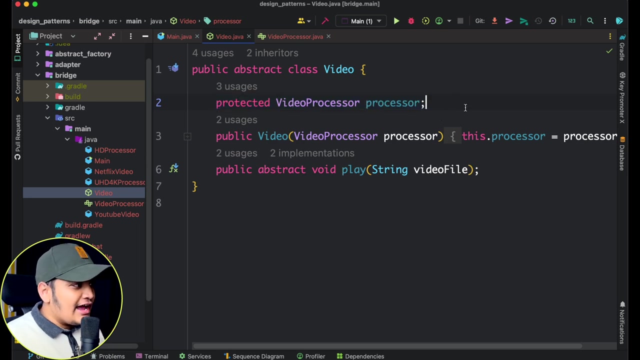 is the separate hierarchy. so video is one hierarchy and video processor is another hierarchy, and you can see that multiple hierarchies we can use using the composition relationship. so that's the idea here. so, within this video class, you can see that i have the object of a video processor. okay, and 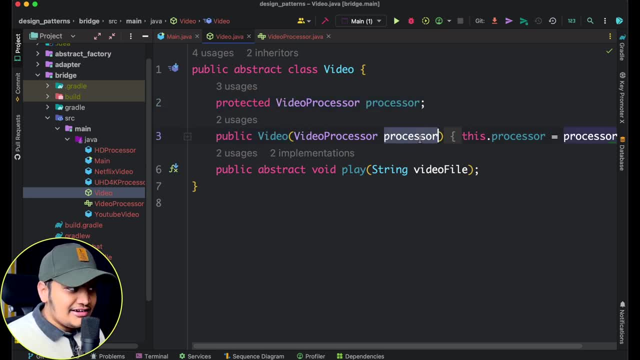 within the constructor. you can see that i am taking the video processor object and assigning the value here. so for this video i have the processor and i have the abstract method play, which will take a video file and it will play it based on the video processor that we have. okay, so? 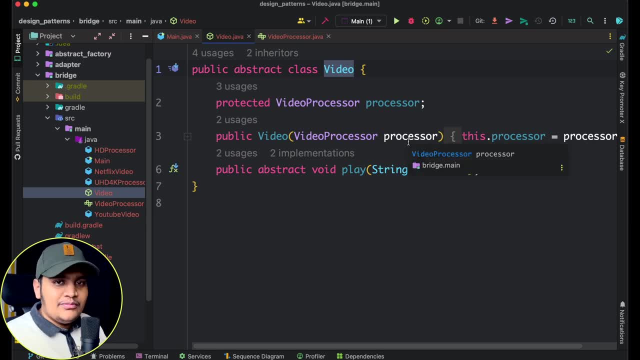 suppose this video have the hd processor, then it will be playing hd. if this video has the 4k processor, it will play in 4k. if it is 8k, it will play in 8k. similarly, now for the video class, we have the abstract method play, which will take a video file and it will 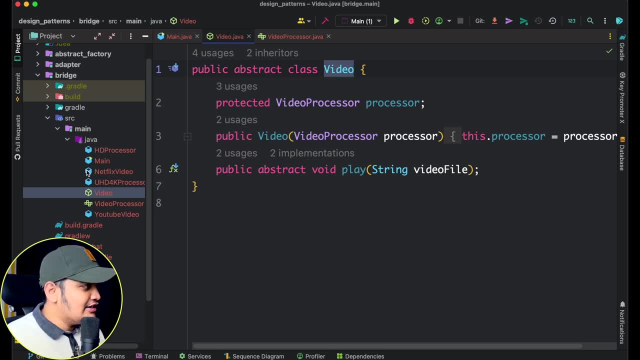 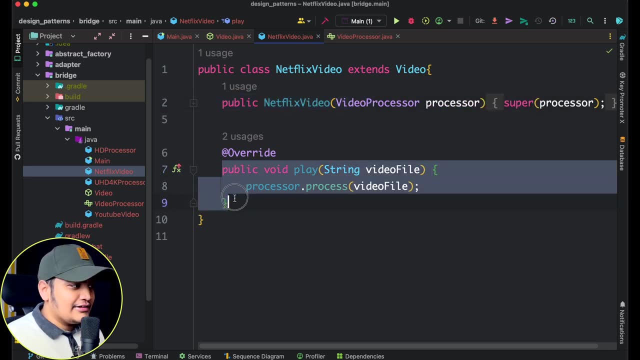 perform this video. okay, we have different classes created. so here you can see that we have a netflix video which is extending video and it has a constructor and it is calling the method play. that this play method will be called and processor dot process. it will call. 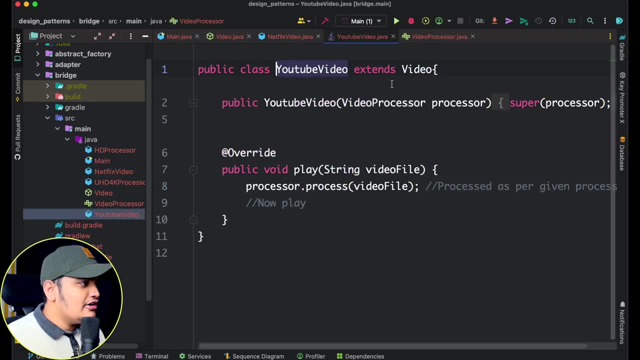 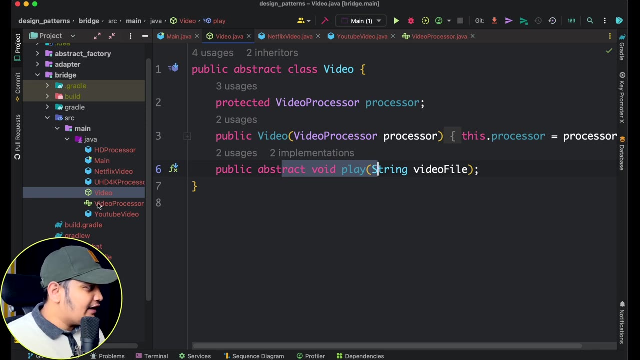 okay. similarly, if you go to the youtube video, youtube video is also extending video and it has a constructor which is taking the video processor and it is implementing this play method. okay, so you can see that whatever we have defined here in the video, that play method we are defining now if you go to the video processor, okay, it. 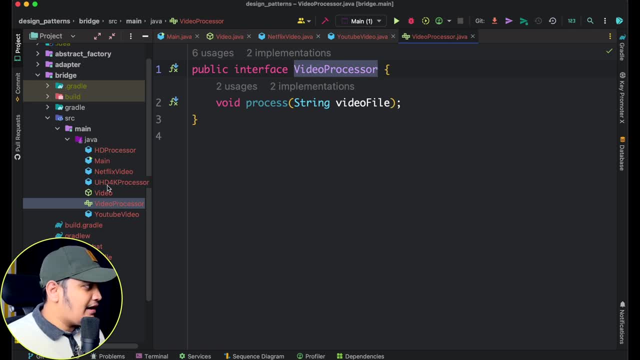 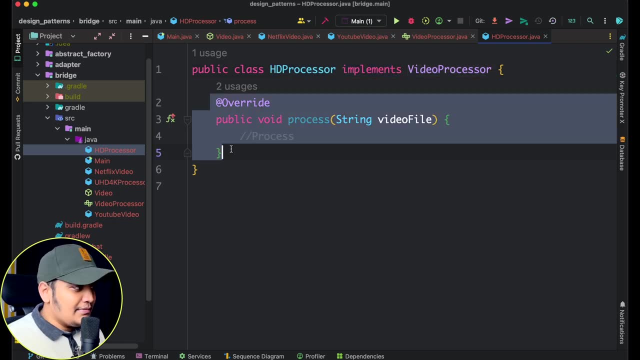 has a process method. so this video processor is been implemented by HD processor. you can see that HD processor is implementing video processor and it has the method implemented. that is the process. similarly, if we go here UHD 4k processor, it is implementing video processor and it is also implementing